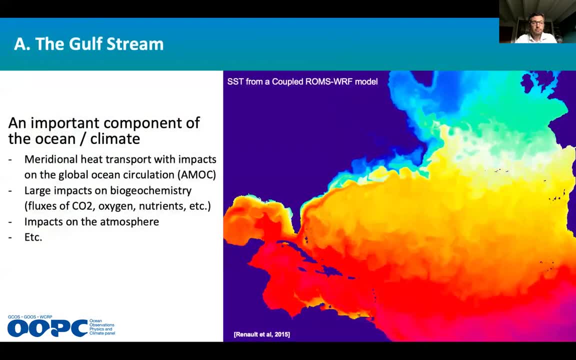 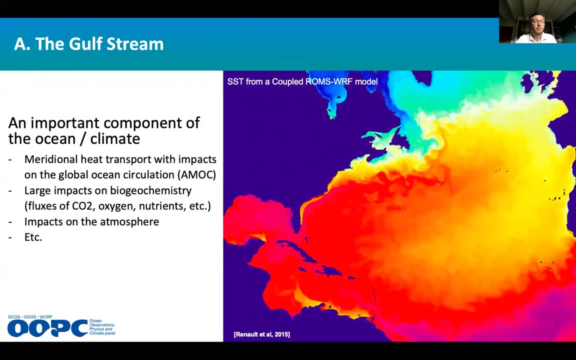 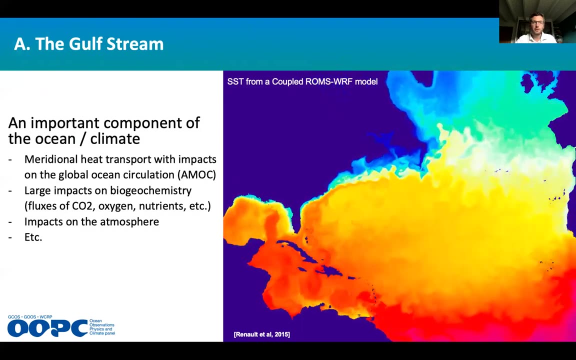 So the goal stream is a Western monetary currents transports heat, salt, nutrient-rich waters forward. You can see an animation of sea surface temperature from a North Atlantic coupled model here. So the goal stream plays a major role in climate. North Atlantic biogeochemistry for the uptake. 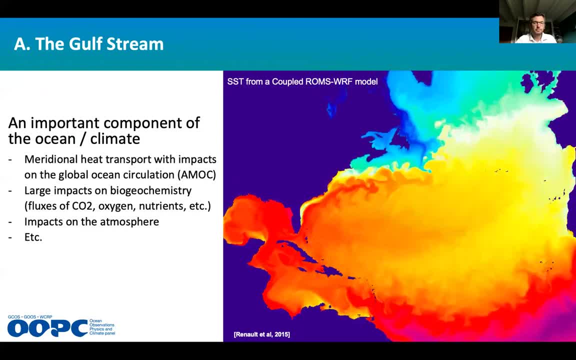 of atmospheric CO2, supply of nutrients, oxygen budgets also impacts the atmosphere Dynamically. it's also a very interesting place because that's where a large part of the eddy kinetic energy of the ocean is dissipated, So it acts as a graveyard for all the mesoscale eddies. 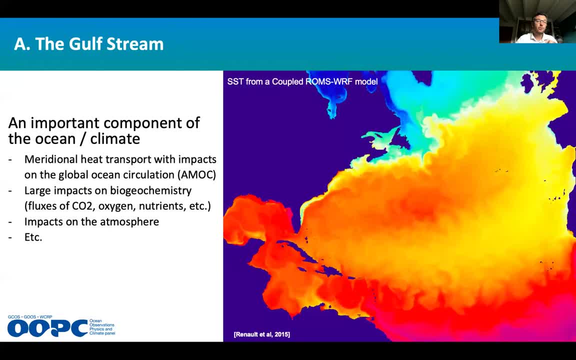 that are generated in the subtropical gyre And these are regions where a lot of small scale processes will have to dissipate energy and also generate mixing, especially along the slope and where we have important topographic features. So the upstream part of the goal stream flowing along the 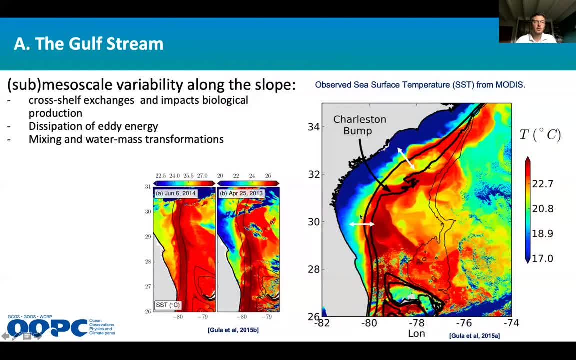 continental slope, so between the Florida Strait and Cape Atras, is also routinely a region where mesoscale- so tens of kilometers wide structures and sub-mesoscale- so kilometer scale structure are observed. These structures play important role for the cross-shelf. 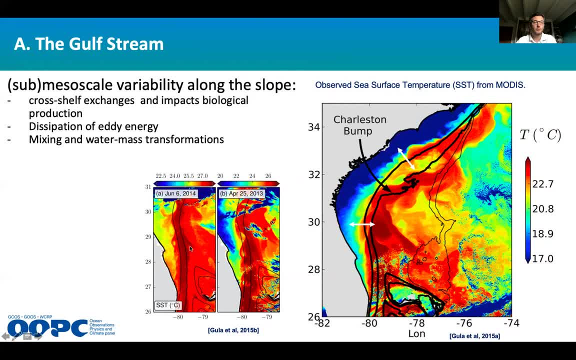 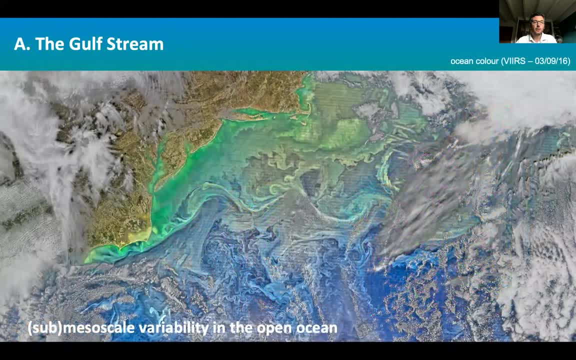 exchange processes, so between shelf water and the stream, with important dynamical, ecological and biological implications. If you look at the goal stream more closely after it's separated from Cape Atras, you'll also see a lot of meanders, goal stream rings and also sub-mesoscale structures. 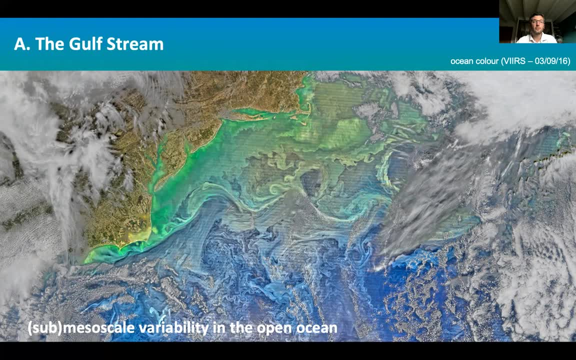 in the forms of fronts, filaments and eddies with spatial scales on the orders of kilometers, So as seen on the ocean color image visible here. So the mesoscale structures have been studied for some time. They are known to generate important horizontal 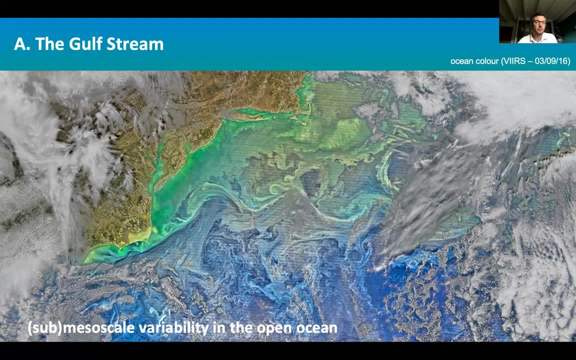 turbulent fluxes with impact on the mean currents and properties, The sub-mesoscale, also have an important impact. So for L-C exchanges, lateral mixing, for example, across the goal stream and also front. they also generate vertical fluxes between the surface. 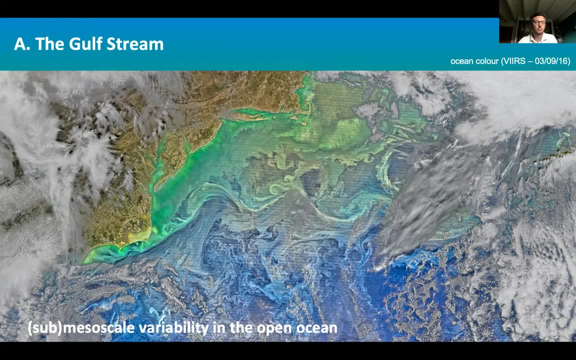 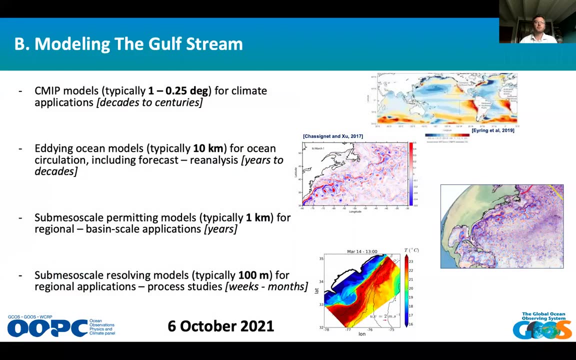 and the interior of this implication for biodegradable budgets, formation of mud waters and other types of applications like this. So there are very schematically different types of models that can be used to model the goal stream. It starts from the. it starts from the. 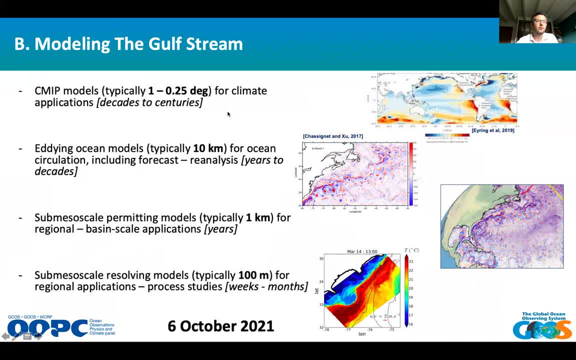 of oceanic components of climate models, So typically the semi models which are used in the context of IPCC reports. These are models with typical resolutions of tens of kilometers, So usually you're unable to resolve the mesoscale eddies, So we talk about eddying ocean models. 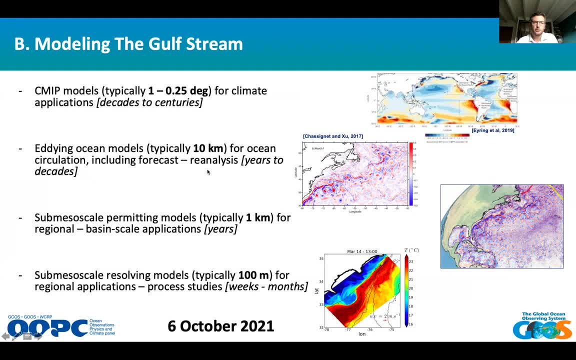 for the one, typically with horizontal grid scales. on the other, 10 kilometer, which are able to resolve baroque instability and the duration of mesoscale eddies and impact on the flow. So these are the models that are commonly used to study ocean circulation with numerous applications. 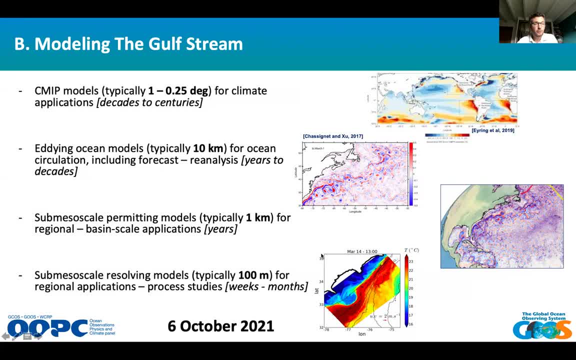 in operational oceanography. Over the past few years we have also seen the development of global or at least basin scale models So able to reach the upper range of sub mesoscale, So with resolution on zero of a kilometer, as that we call sub mesoscale, permitting. 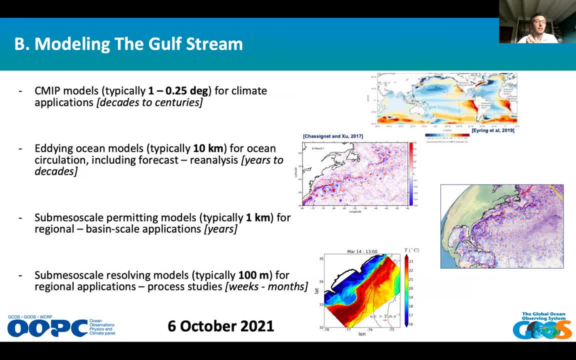 And finally, we have limited extension domains, original models which can be sub mesoscale permitting as well or sub mesoscale resolving, when we go to hundreds of meter or less, And these are very useful for original applications, process studies and a wide range of applications. 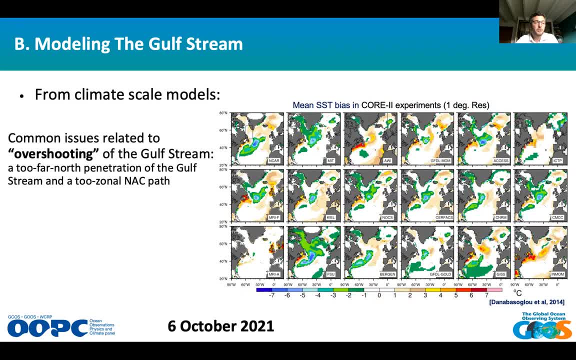 So the Gulf Stream is notoriously difficult to model, especially for climate scale models. A well-known issue present in many of these models is the overshooting of the Gulf Stream, For example. in other words, the Gulf Stream doesn't separate where it should. 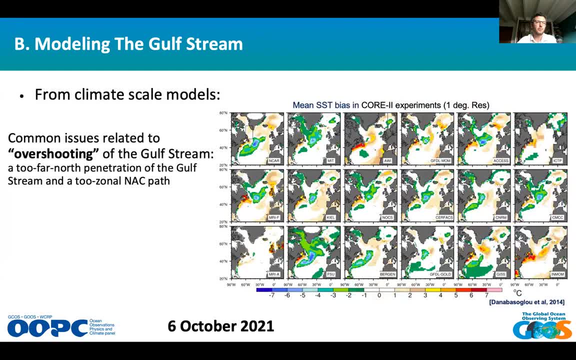 at Cape Atreus, but it just follows the continental slope and penetrates too far north. This is very common in models, as you can see on all these panels showing mean SST bias in one degree experiments. So as it separates too far north. 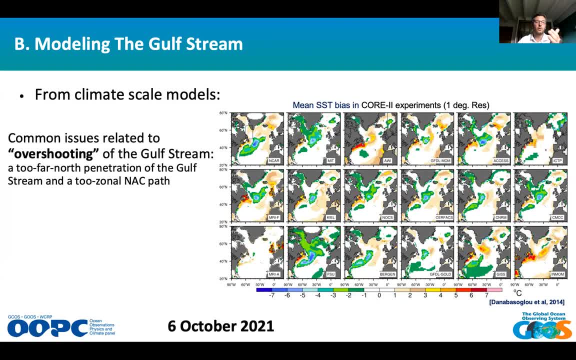 it induces a strong positive SST anomaly north and negative south Also have implications for the North Atlantic current downstream And so this strong temperature anomalies generate systematic SST biases with implication for the atmosphere, weather precipitation over Europe. so many problems in climate models. 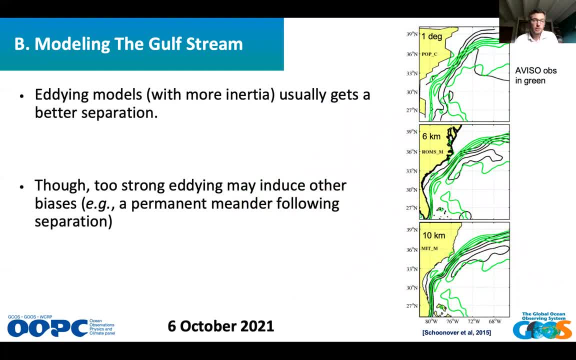 This problem is often solved by increasing the resolution, diminishing the effective viscosity to get a more inertial Gulf Stream. So then usually dissipation becomes more realistic. You can see an example of that on the figure. You have an example of that on the figure. 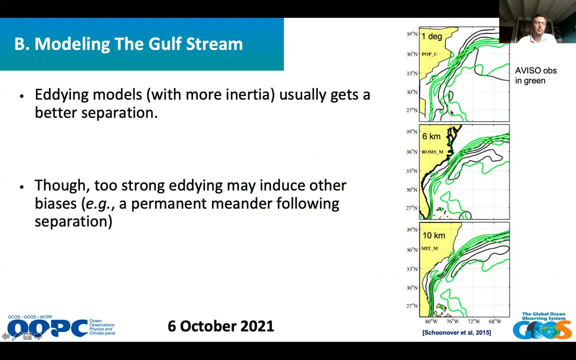 You have an overshooting model. You see the contours in black here on the upper panel compared to the observations in green. so how it should be. So this is strongly improved when we get to heading models with six and 10 kilometers here. 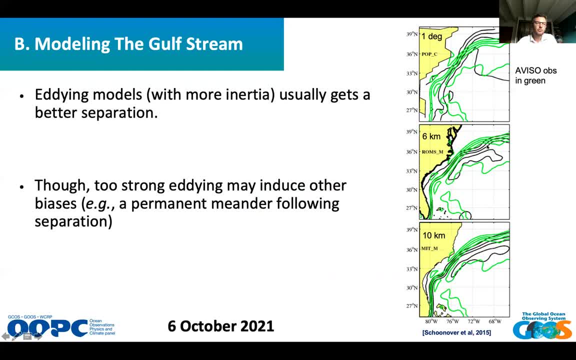 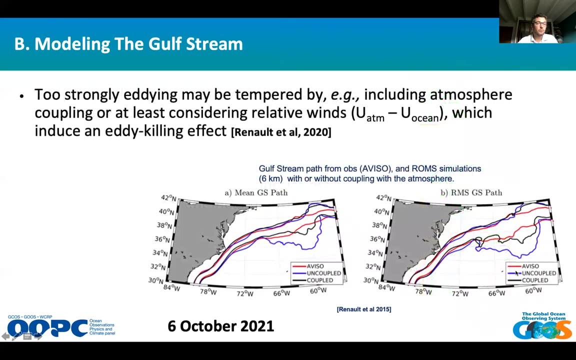 However, you can see an interesting fact that in this case we get a small bias in the form of permanent meander just after separation. here, which is common in models where we have a bit too strong AD activity, And this can be resolved, for example, by removing energy. 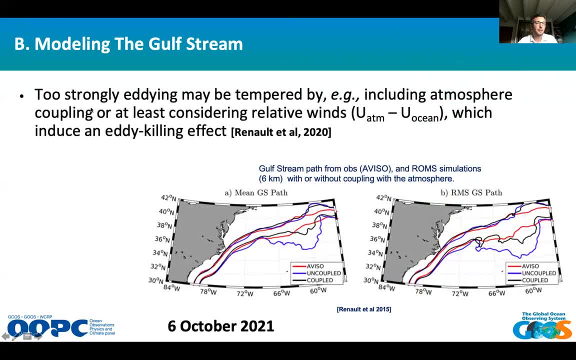 So in this case it was resolved by adding atmospheric coupling or just considering relative winds in the ocean force model, Relative winds meaning the difference between atmospheric winds and ocean currents to complete the stress at the surface. This has an AD claiming effect: Remove 20% to 30% of the AD kinetic energy in this region. 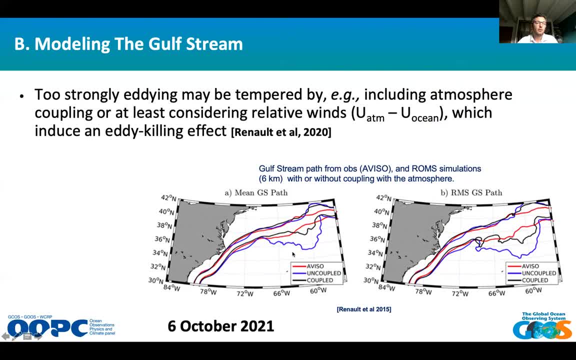 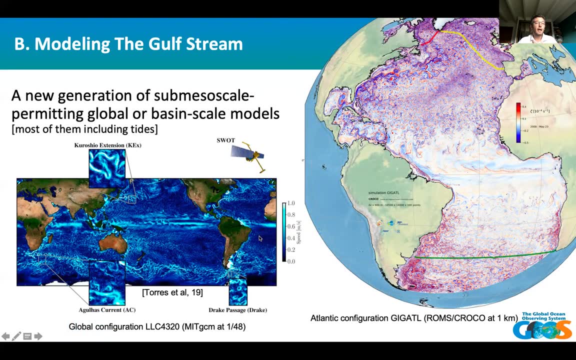 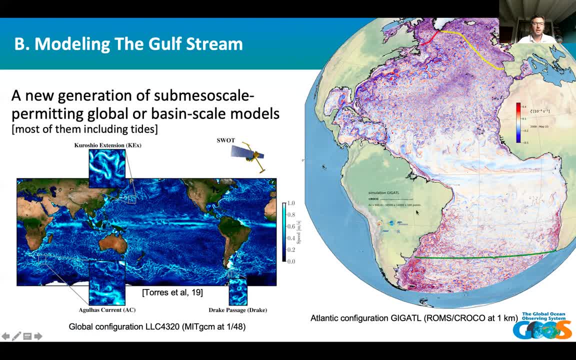 which is what is done in most models of this of this time, also has consequences on circle stream meandering and viability. so typically resolving sub mesoscale may induce upscale energy transfer and energize further mesoscale eddies in some region. in others you can also have 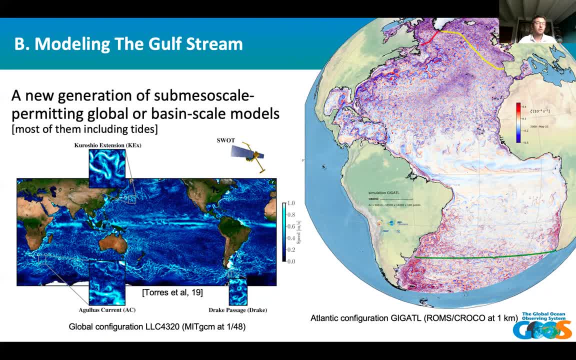 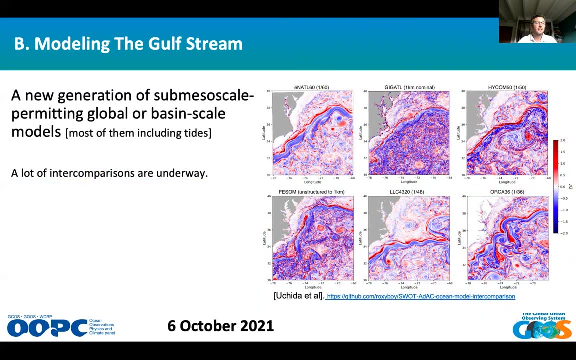 internal waves acting to extract energy from the eddies. so you are adding new pathways for energy and modifies the mean structure of the flow in many cases. so there are. there is a strong effort currently to intercompare the different type of models of this, of this type you can see. 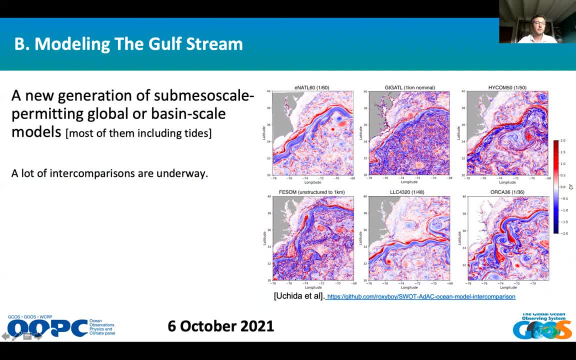 examples here showing a snapshot of vorticity in the gosium region for six of these models. the interesting thing is that they are all using different type of numerical options: vertical coordinate, subway scale, turbulence parameterization, addictive scheme, etc. so it is very useful to to compare them and see differences in. 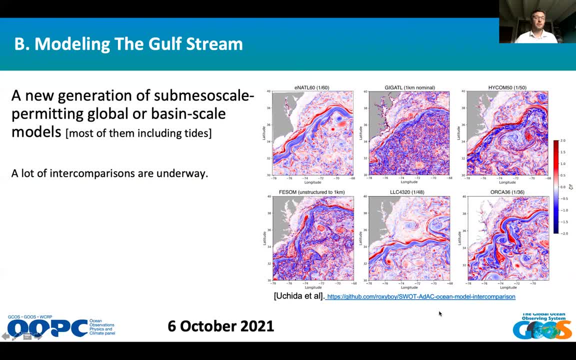 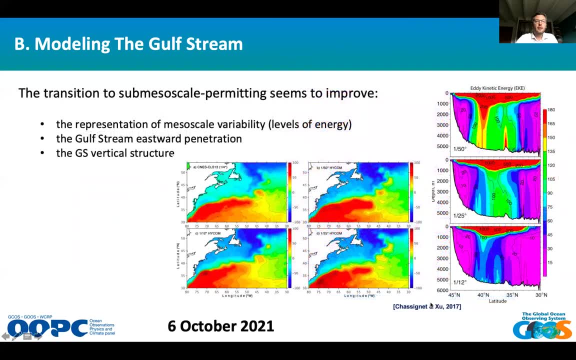 the are the differences in the setup translated to differences in the statistical properties of the object. some works. i've already shown that for some of these models at least, the increase in resolution was leading to a more realistic structure of the goal stream. you can see an example here of icom simulations going from the 12th degree to 50th degree, where the viability is. 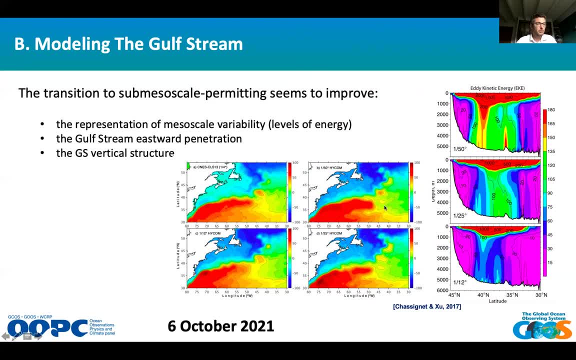 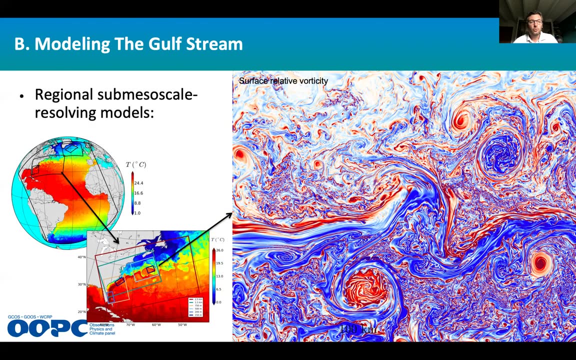 expected, and it leads to a more realistic eastward penetration of the goal stream and also more realistic vertical penetration of ek and more realistic vertical structure of the current. so then, you can also go further by using sub mesoscale resolving models, so usually over much more limited regions and and for for smaller periods, particularly months. 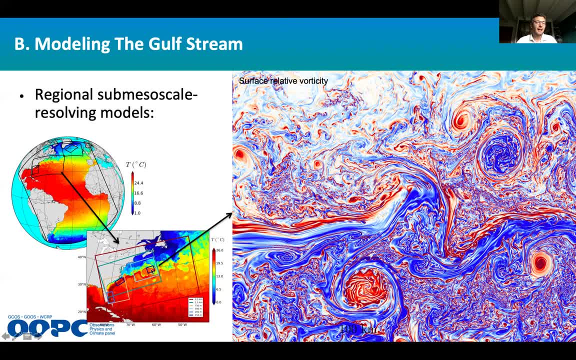 or years later, even in the early 20th century, and so on and so on. this can be done by nesting irration model high resolution models into lower resolution ones, by in scale solutions or realizers. you see an example here of the vorticity snapshot of the goal stream after: 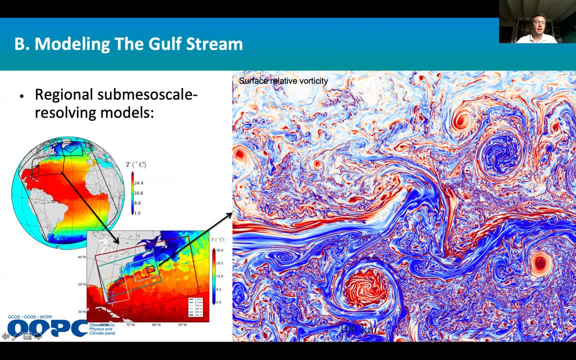 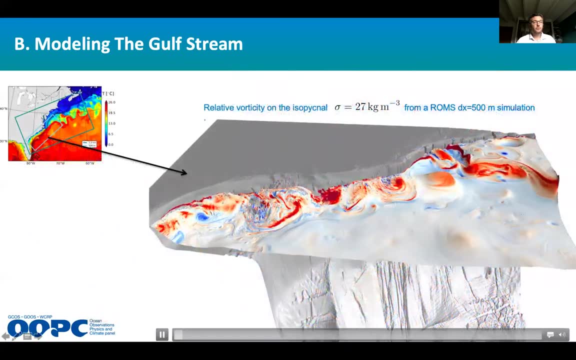 separation uh with even more intense sub mesoscale fronts, uh filaments and associated vertical velocities, and it doesn't really show signs of convergence yet. so we know that properly model this kind of scales. There are also important small-scale processes happening at the bottom of the ocean, so especially where the current interacts with the topography. 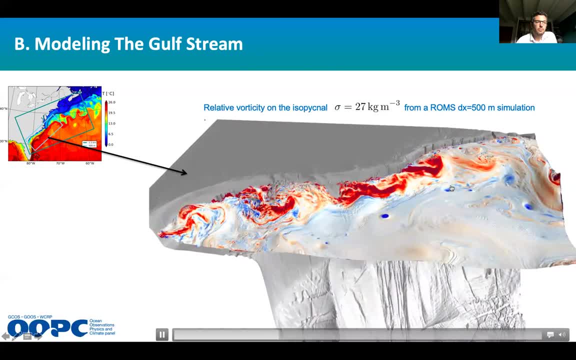 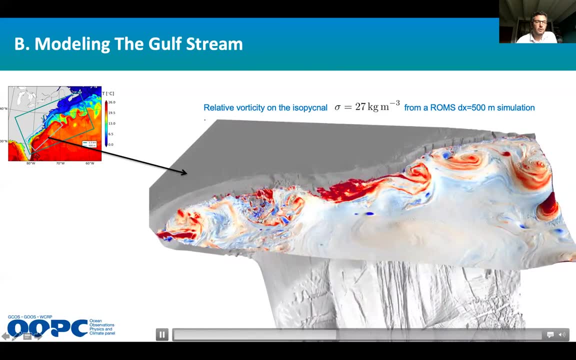 You can see an animation here of the Gulf Stream flowing along the slope. The colours are showing relative velocity and the surface corresponds to one isopic node in the model. It shows in particular a turbulent wake on the lee side of the Charleston bump, which is a 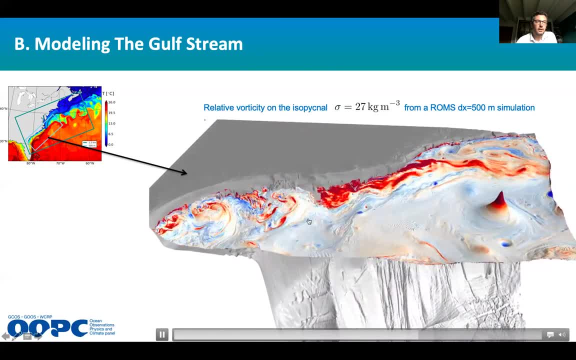 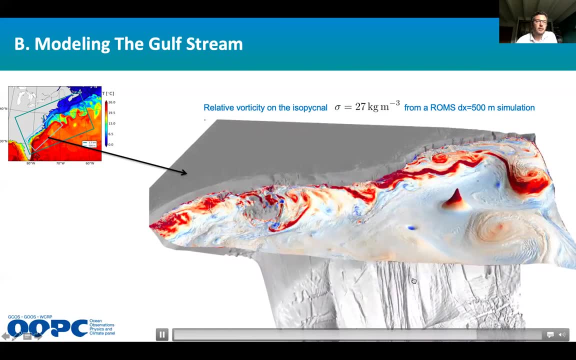 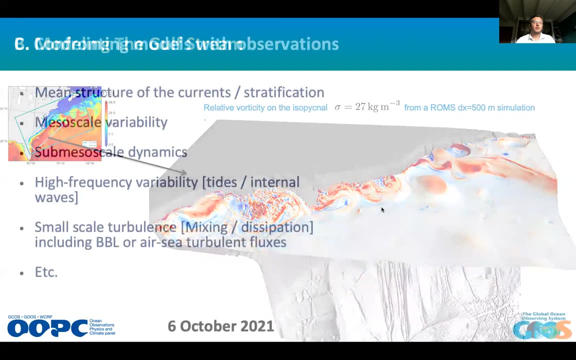 grey area here, outcropping the isopic node at this location, A generation of more sub-mesoscale eddies or mesoscale eddies in the flow. So you see that models are trying to get more and more realistic. so at least they are trying to get more and more realistic. so at least they are. 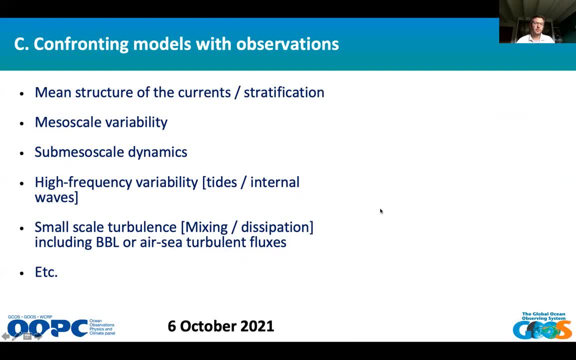 trying to get more and more realistic. so at least they are trying to get more and more realistic terms of processes included in the physics of the model And they're going to finer and finer resolution. But of course these models are far from perfect by definition and they need to be. 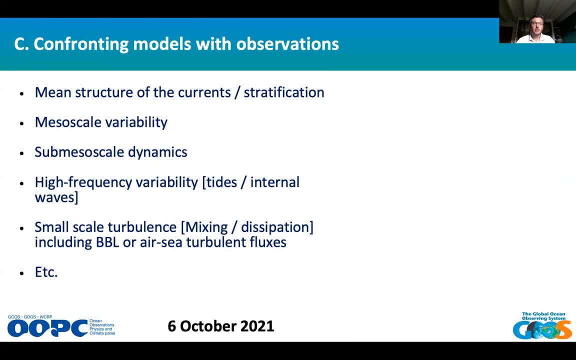 constantly confronted to observations, First to be validated, to be sure that the physics numerics are doing a reasonable job at least, And then eventually, observations can also be used for data simulation, so to constrain the the model, or even to construct parameterizations for processes that are not resolved by the models. 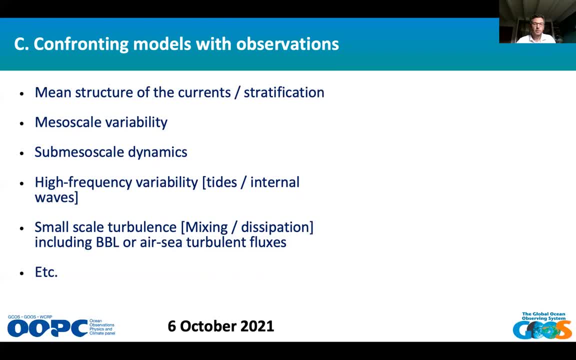 So what you validate in the model really depends on the objectives of the model and the spatial and time scales that are targeted. So it goes from the mean structure of the currents: mesoscale viability, sub-mesoscale properties, high frequency activity. so what happens related to the internal waves and tides, and even the small. 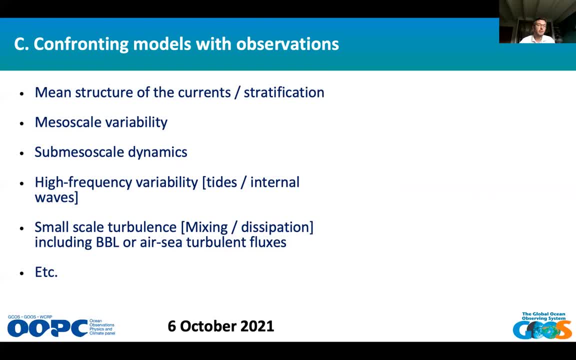 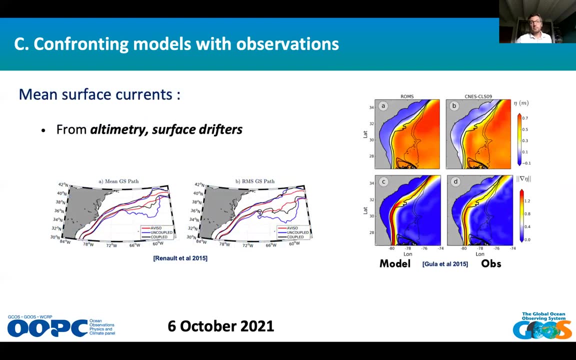 scale turbulence, So, in particular, what's happening in the bottom of the layer or in the surface layer and related to RC turbulent fluxes. So, basically, the question is: which type of observation can we put in front of that? One of the most useful data sets is, of course, altimetry. 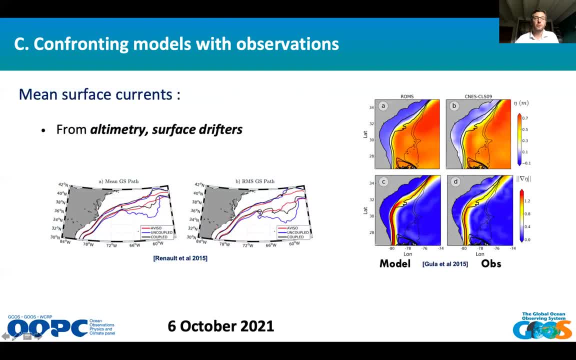 If you are interested in mesoscale and larger, you want to monitor the path of the gold stream, like in the figure here. this is how it is usually done. Unfortunately, the effective resolution of altimetry is on the other, almost 100 kilometer, let's say, and it's also not always variable- near. 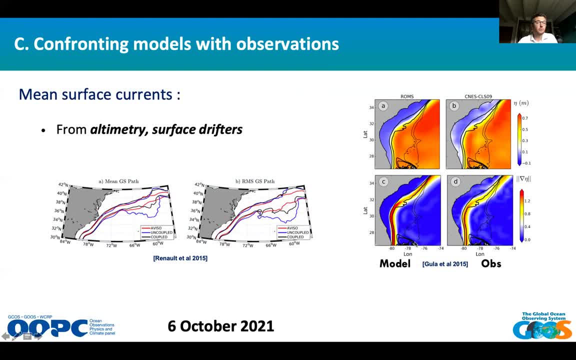 the coast. So, for example, you cannot get the full amplitude of ssh radiance for the gold stream when it flows along the slope there. So this type of data can also be combined with drifters, so there's a growing global database of drifters that can be used to help mitigate this kind of issues. 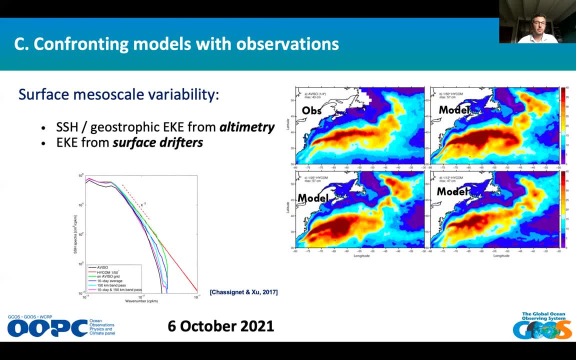 Thinking about mesoscale variability, the same data can be used. So maps of ssh variability or eke derived from that can be very useful to compare the different type of models and assess their realism. So of course, altimetry corresponds to scales which are: 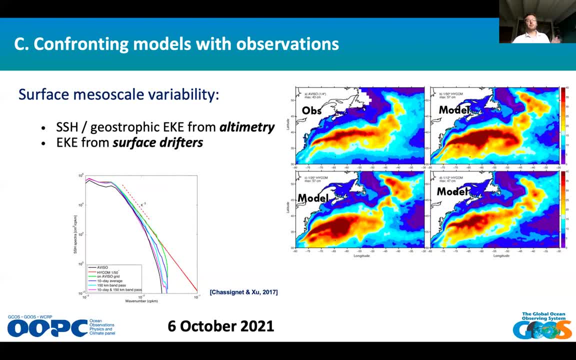 on the other 400 kilometers, time periods on the other 5 to 10 days, and models usually have to be smoothed out to get to the same spatial and temporal resolution to get to make up for a fair comparison between the two. You can see, for example, what happens here if you compute a. 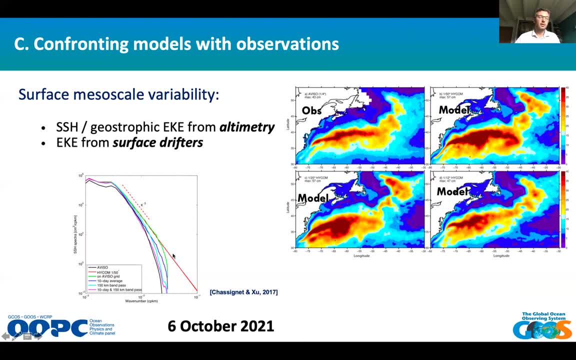 spectra for ssh variability in the model, you get something much stronger than in observation. But if you smooth out using a 10 days period and the bandpass filter of about 150 kilometers here you get to something which is pretty, pretty similar. So hopefully the new satellites like the SWOT. 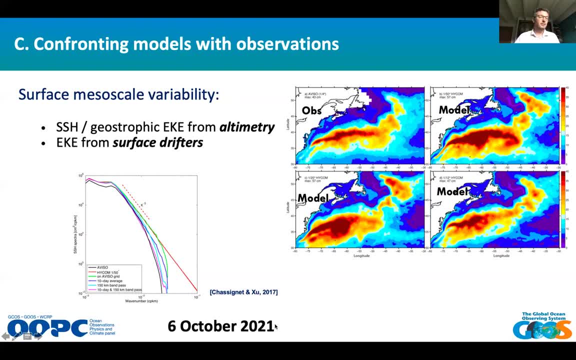 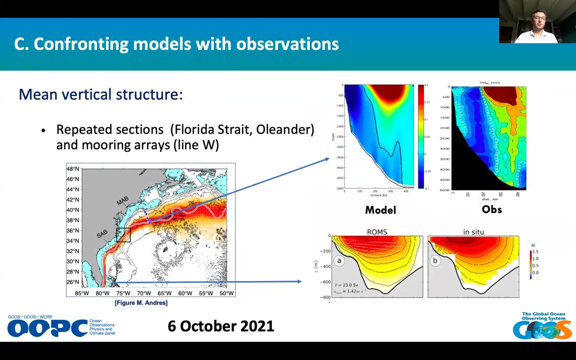 satellite will help provide information at these smaller scales, even if, of course, the time sampling will still be an issue. If you are interested in what's with what's happening below the surface, it's even more difficult to check the realism of the of the model. So the vertical structure. 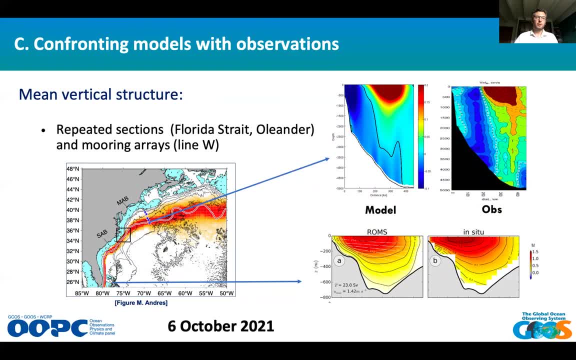 of the currents. we don't have a lot of data to compare it with. If you have seen the previous talk by by Magdalena Andres, you've seen that there are a few repeated sections, like the one in the Florida current. here They are moving lines like line w, and these are typical examples of what you can. 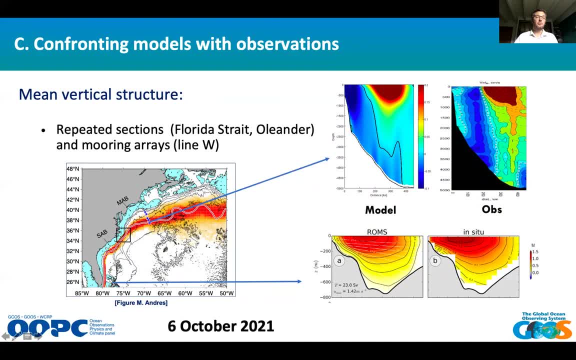 compare between model and observations But unfortunately there is not a lot of data between these lines in terms of repeated sections to get the mean structure of the current Despite the strong changes happening in the structure and variability. there's a version between these two sections. 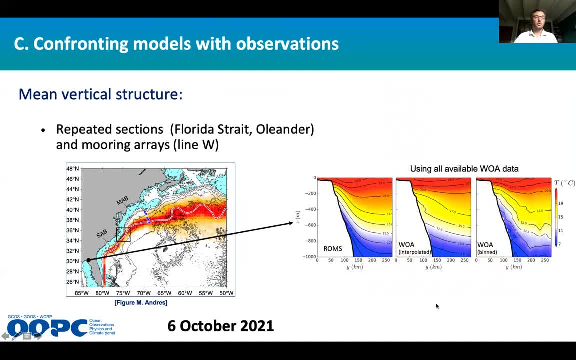 As a quick example. for example, if you just use all the available TS data from the World Ocean Database, you can construct a mean temperature profile here. So if you use interpreted data, of course it's a problem, because the gradient is smoothed out. 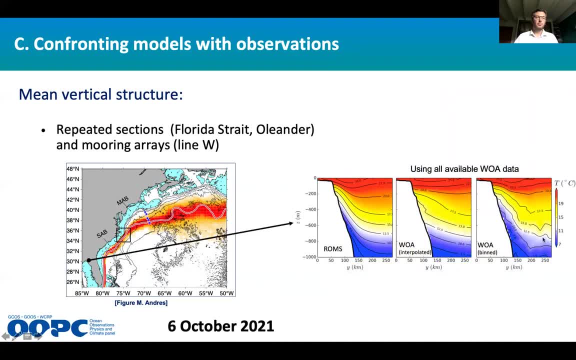 But if you just bin all the available data- so more than 50 years of data- you start to get something, something decent. And it's possible in this location only because the current is mostly flowing along the slope, not meandering a lot, because if you do the same thing after separation, 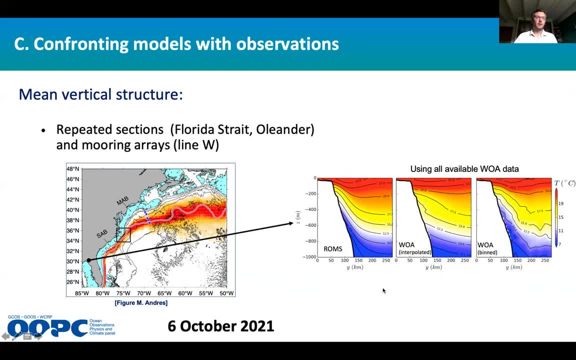 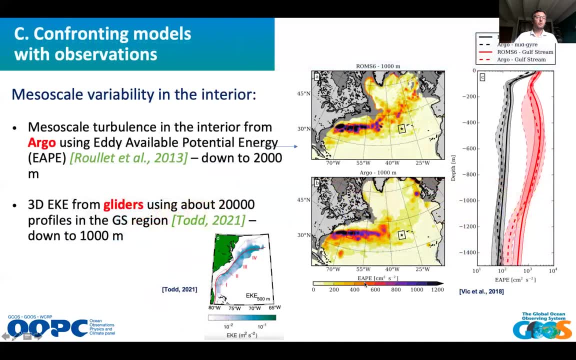 you'll just be completely smoothed out because of the meandering of the current. So now, if you also want to quantify the mesoscale variability in the interior, below the surface, it's possible at least down to 2000.. So now, if you also want to quantify the mesoscale variability in the interior, below the surface, it's possible at least down to 2000.. 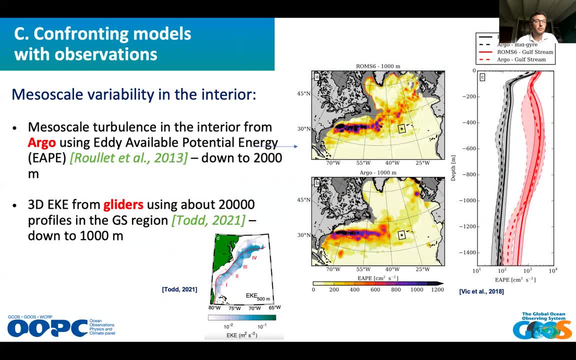 meters. For example, you can use observation from the Argo floats compute diagnostics such as any available potential energy. This is something related to the vertical displacement of isopignols, and comparisons between models and this Argo dataset are very useful to provide. 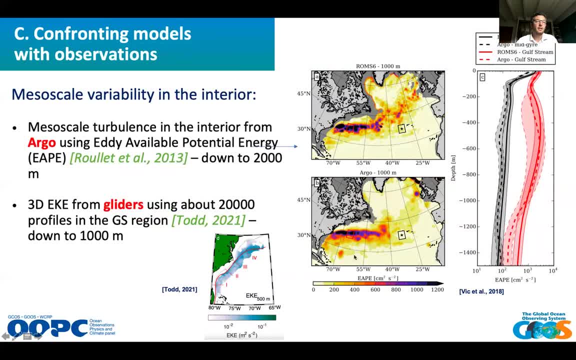 some vertical structure of the mesoscale variability and help characterize different types of regimes. More recently, data from the GUIDOS program have also been compiled to come up with mean and the eddy kinetic energy over the first 1000 meters in this region, where 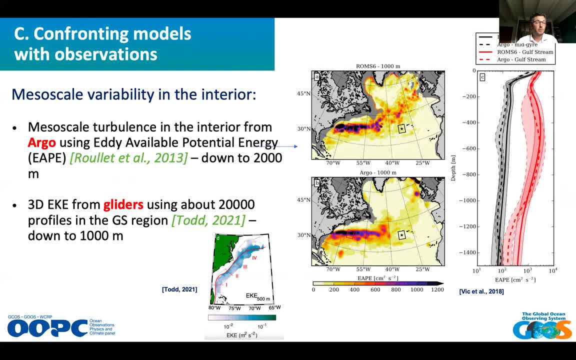 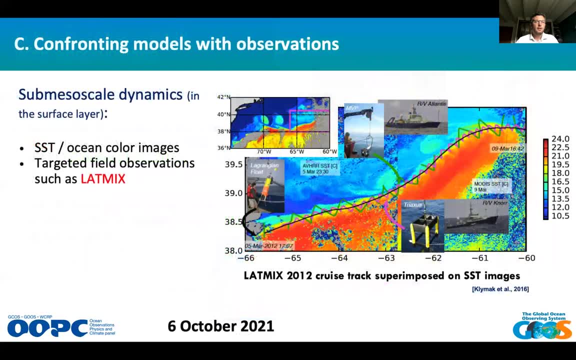 the golfram is flowing along the slope, So this is a very useful dataset that can be used to compare with models. So when it comes to even smaller scales than that- the sub mesoscale- it becomes even more difficult to find data with enough spatial and time resolution to come up with useful statistics that can be. 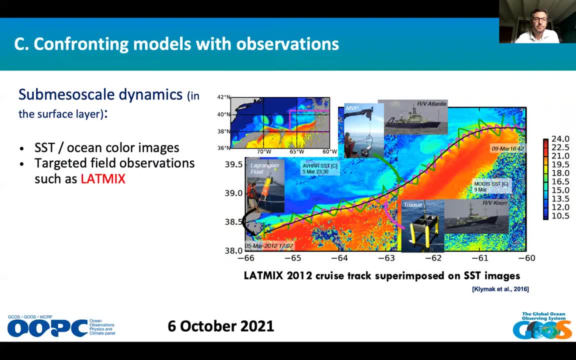 compared between models and observations. So SST ocean core images are showing a lot of nice features at the surface at small scales, but they cannot be used to infer the dynamics of velocities, for example. So our knowledge comes mostly from dedicated multi-instruments experiments. 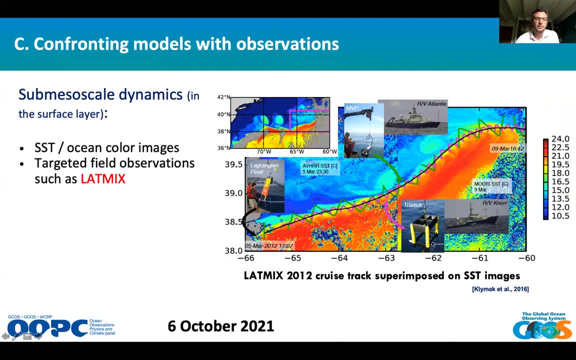 such as the LATMIX-1, whose design is shown here. So this type of experiments typically use several shapes, a lot of instruments and focus on a specific region. Here's a north wall of the Gold Stream, in order to provide a lot of high resolution simulations at the same place. 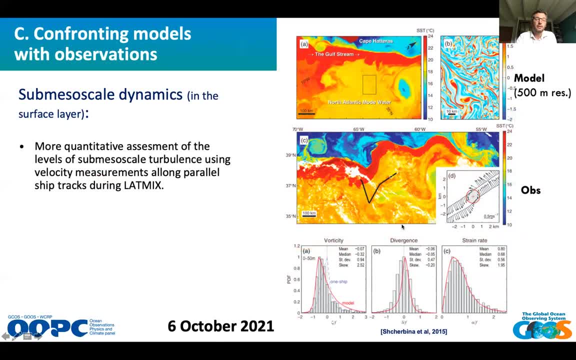 And one of the very interesting experiments in terms of model validation that came up with. that is an experiment where two shapes were used in parallel, as you can see, in order to provide 2D velocity gradients so that you can get statistics on the vorticity divergence. 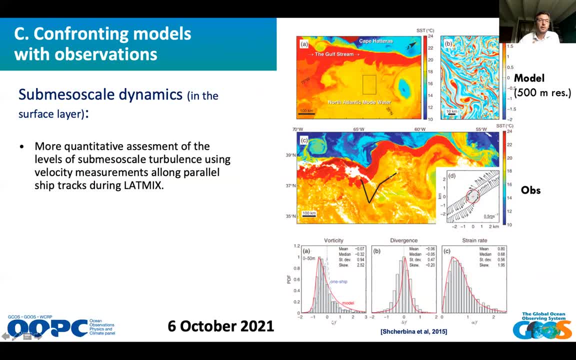 and strain distributions in the field. So if you compare the same statistic from the model that you see on the top panel, from these observations here, you can see that you get distributions in fairly good agreement. So histograms are observations, the red curves are the model. 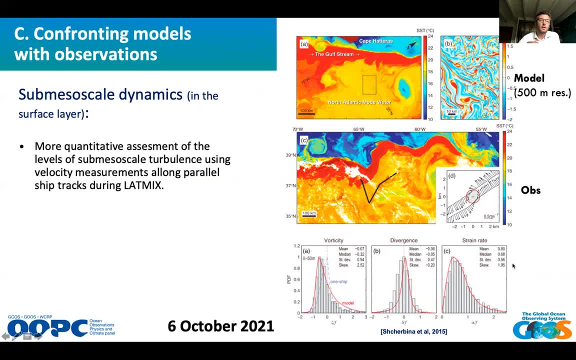 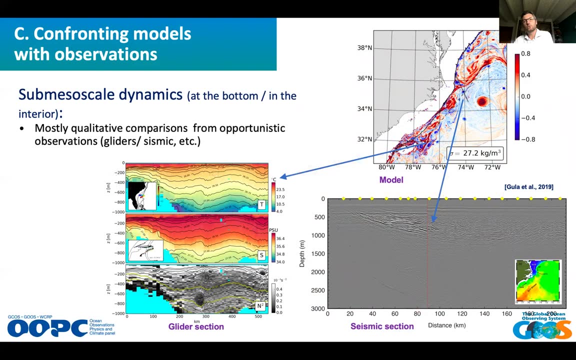 So this is one example of a very successful comparison at this scale, but it is really one of a kind. So if we go deeper below the surface, as you can imagine, it's even more difficult to get observation. with fine enough spatial coverage and time sampling, You can get glider sections. 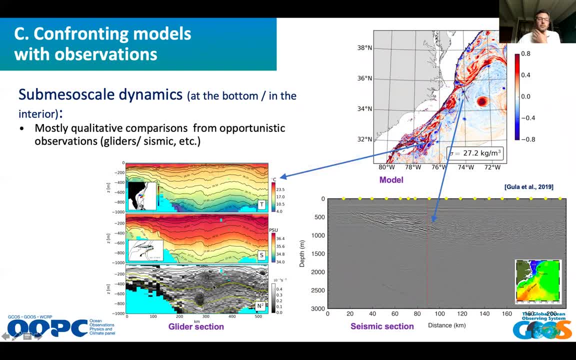 in the upper 1,000 meters. that provide kind of snapshots of the pretty small scale structures. For example, here you see a model on the panel showing the formation of small scale eddies, So we can make qualitative comparisons with gliders, because we 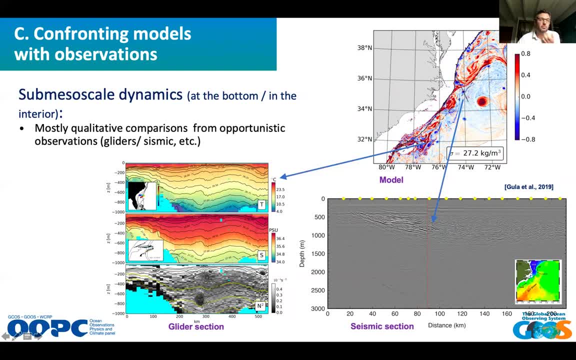 see the same type of structures, not exactly the same at the same place, but just the same class of structures. We can find the same things, for example, in opportunistic seismic measurements, which shows a fine scale, vertical gradients in temperature mostly. 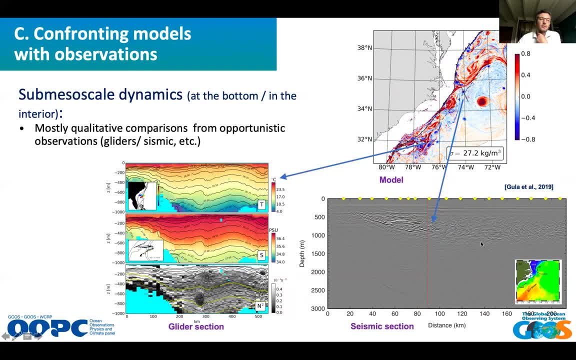 But this is really qualitative and it's difficult to get something more quantitative when you talk about this type of structure. But if you go deeper below the surface you can see that this is a very good example of this type of dynamics and structures. 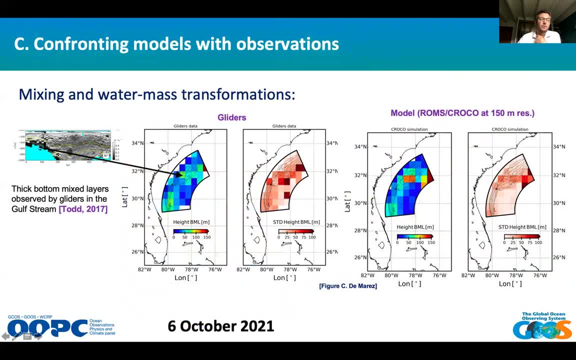 So, especially as we know that, close with topography, a lot of important mixing processes are happening. So one way to map this, for example- and gliders have been used to do that- were to measure the thickness of the bottom monorail layer with the gliders. 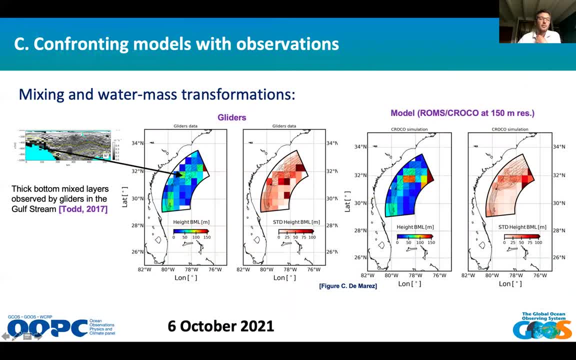 This can provide a map that you can see here, with the mean and the variability of this bottom monorail layer depth. This is again another diagnostic that we can compare to models. In this case, a very high resolution model of the region is doing fairly good in terms of producing that, but it's difficult to. 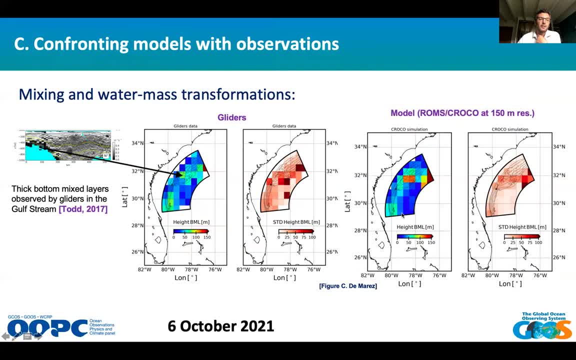 go further in terms of comparisons and validation for this aspect Especially, the mixing itself is very difficult to quantify and to observe And we know that it is an area where models have flows and and it's very difficult to check how they're doing and try to improve this aspect. If we look at 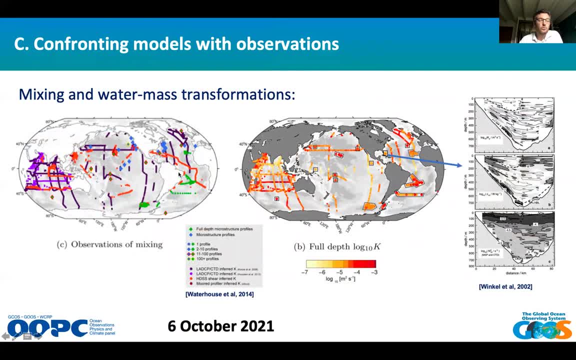 specific microstructure measurements, so to measure the small scale, dissipation and mixing. we don't have such a large number of direct measurements Globally. we don't have a lot of measurements and the Gold Stream, despite its importance, is no exception to that. 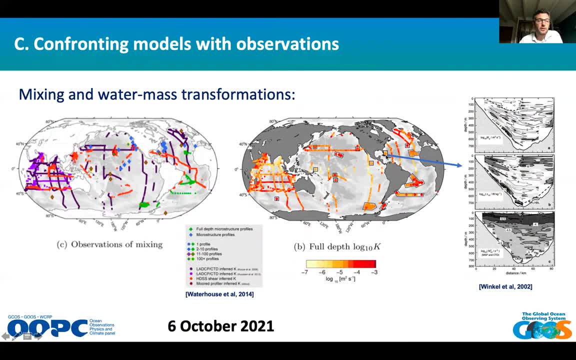 We have a few microstructure measurements in the Florida Strait Again. you see here some examples on the right. We also have some data along the sections. this is a Hollander section, I think, But these are not microstructure measurements but 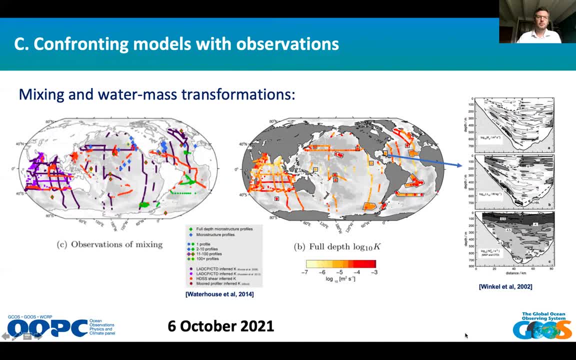 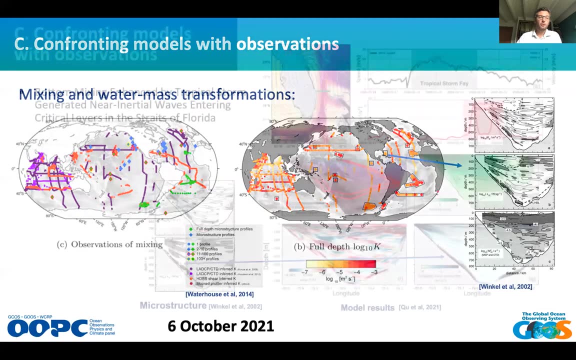 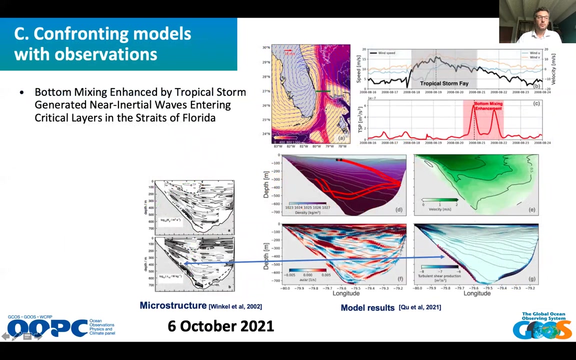 data which are inferred from CTD and ADCP. So we need to better understand what's going on, especially between the Freudian strait and the section which is downstream of separation. So, for example, recent work has highlighted that some of the mixing in the Freudian strait 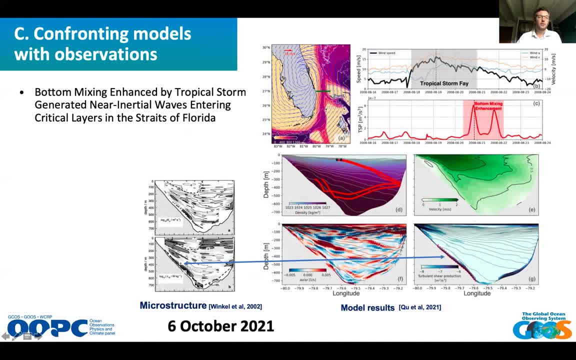 for example, the band of eye mixing you can see on the Western slope here can be reproduced in idealized and realistic models when we take into account tropical storms, generation of initial waves. This initial wave propagates- oops, sorry- in the flow. 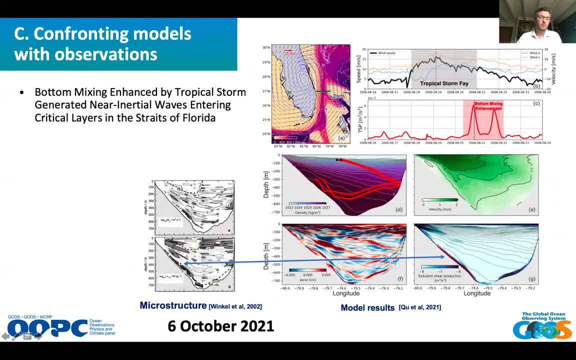 can be reflected on the Western- sorry, the Eastern- slope, And then they can focus into the critical layers that are formed here, where, as the big nodes are more or less following the continental slope And they are trapped here and generate this strong mixing. 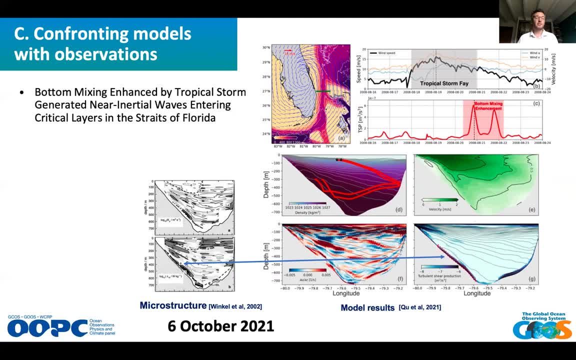 And there are presumably other type of processes, more scalability, instabilities, leeways, for example, especially at the Charleston belt, that are acting to generate mixing and in the middle of the stream And that can induce water mass transformations. But we don't know much about this from observations. 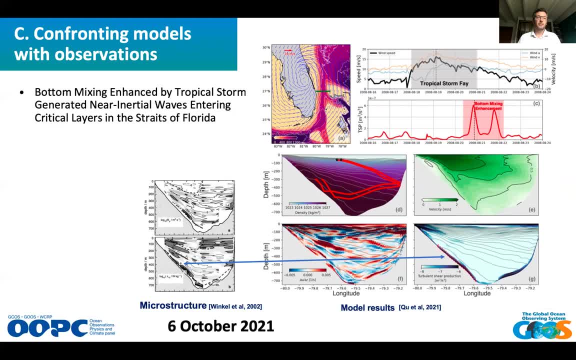 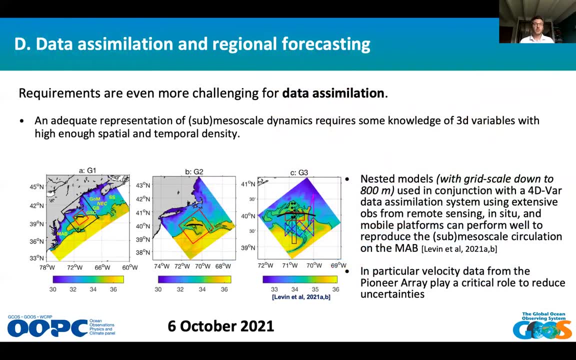 And it's difficult to evaluate models on these aspects. So when it comes to data simulation, everything becomes even more challenging. So we have barely enough to compute long time statistics on meso, sub-meso scale processes. So getting enough 3D data and resolving the time. 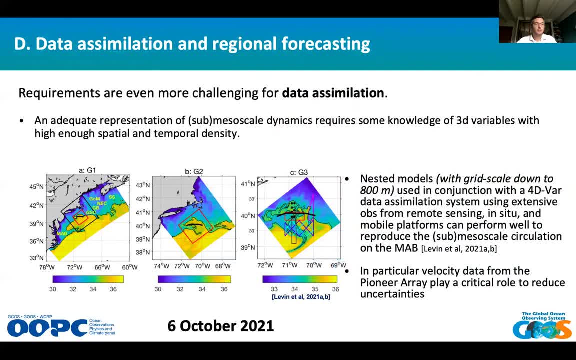 and spatial escapes involved is even more complicated. There is a nice example shown here of high resolution modeling and data simulation on the mid-atlantic bite at the location of the pioneer array, so where a lot of data are available, And it manages to reproduce fairly well the circulation. 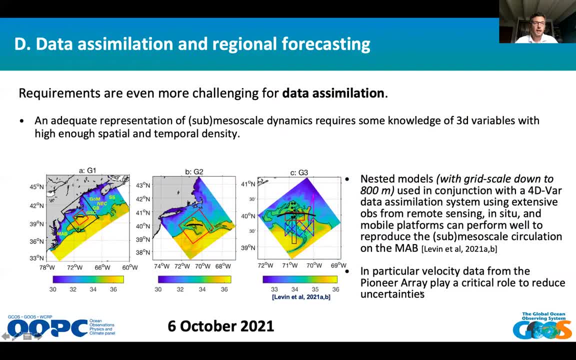 even at some mesoscales, And it has been shown that in particular the velocity data from the pioneer array played a critical role uncertainties in the production of the circulation. So this doesn't come as a surprise that 3D data with high enough resolution 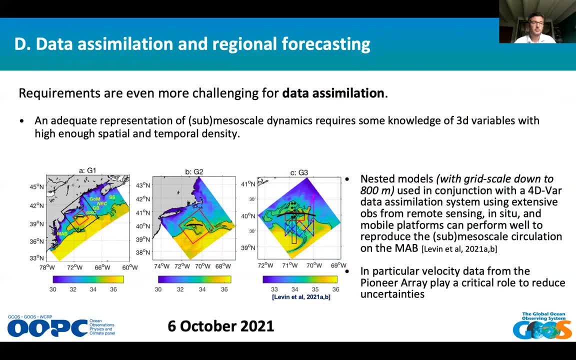 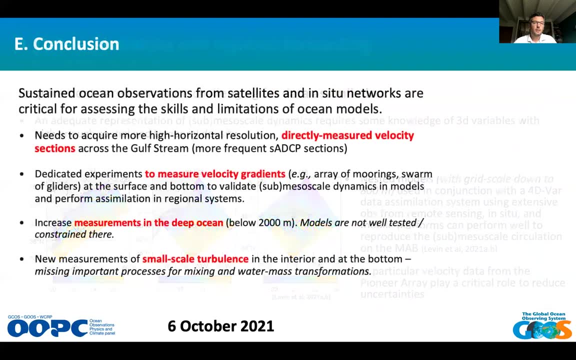 in particular, velocities are needed to do that, But it's again reinforcing the point that we need to get as many of this data as possible to be able one to evaluate the models and also to perform a data simulation, at this case. 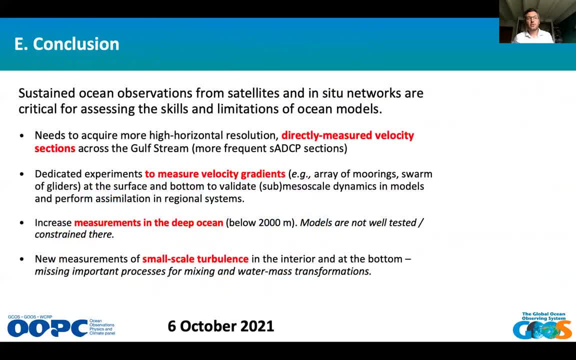 So in conclusion, I will just stress again the importance of ocean observing networks for improving ocean circulation models. These sustained observations from the satellites and the networks are really critical to routinely assess the skills and limitation of the circulation models over time scales ranging from hours to decades. 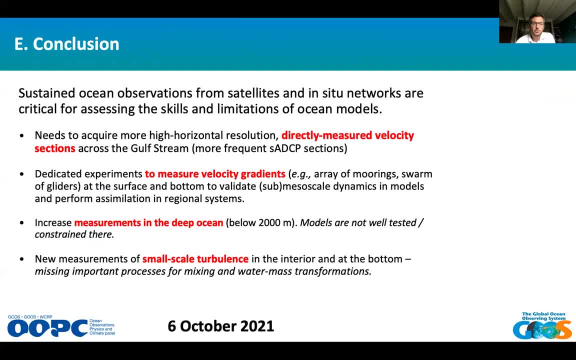 So I will just repeat some of the recommendations made in the first talk, especially pertaining to the need for more frequent direct measurements of velocities with high enough resolution in different places of the observable stream, Ideally also experiments designed to measure velocity and trace aggregations at meso.